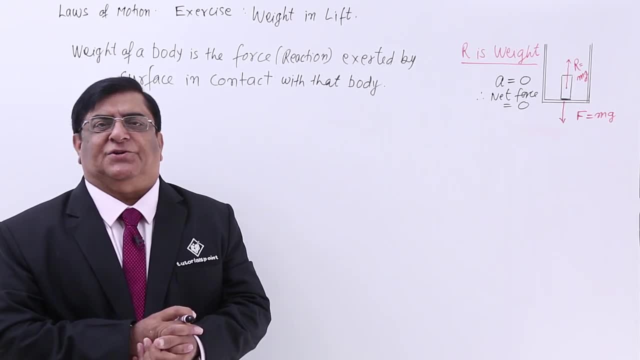 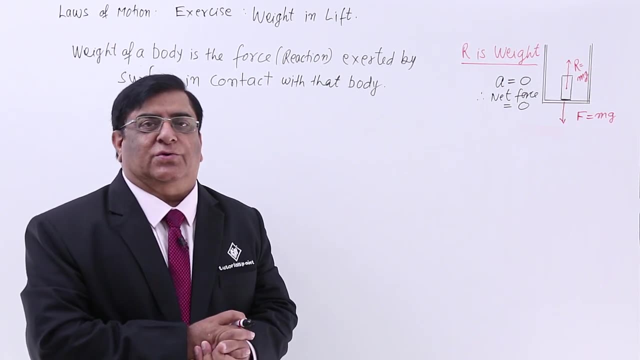 We will do one very important exercise now that is related to weight: Weight of a person, weight of an object. First, what is the meaning of weight? So in physics there is a separate meaning, different meaning, which we are supposed to understand. 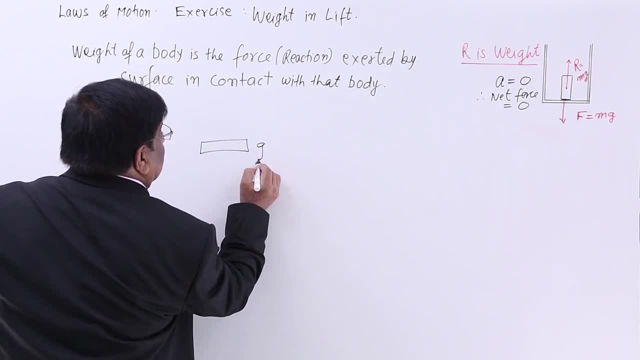 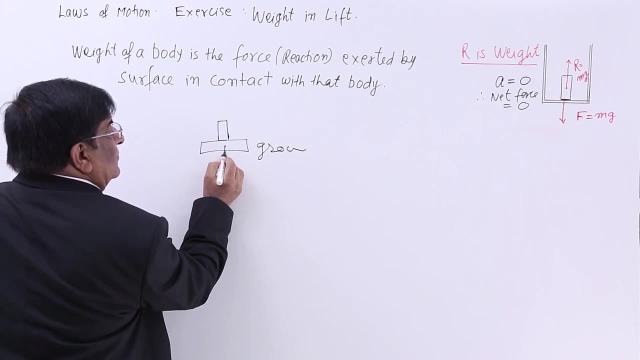 If I am standing on the ground- here is ground and I am standing on it- then I am pressing the ground. I am pressing the ground with a certain force and I know that force is mg. If I press the ground, then ground does not move. What is happening to my force? Answer: the force is balanced by the reaction. 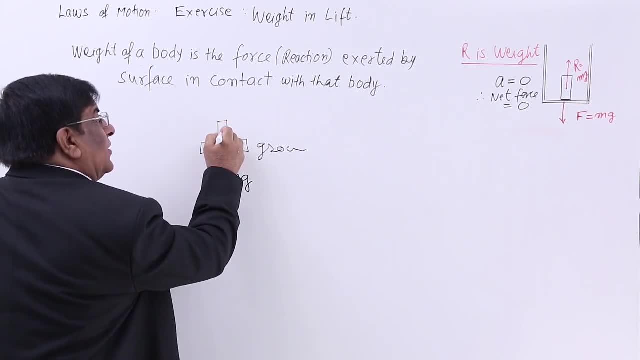 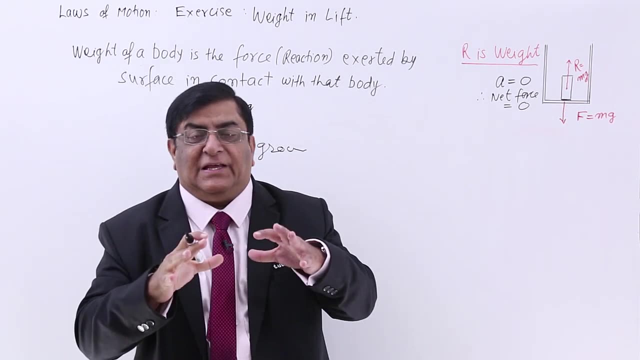 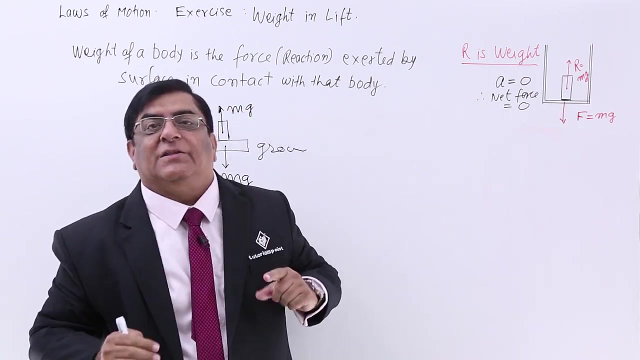 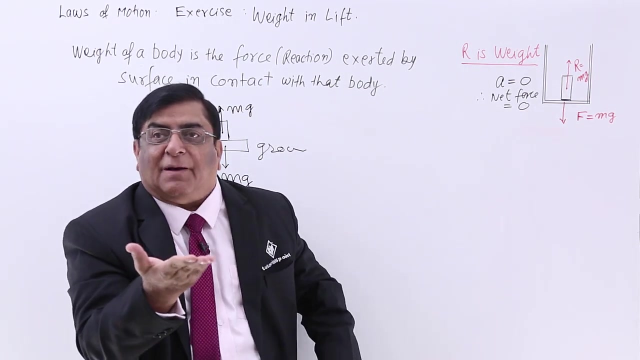 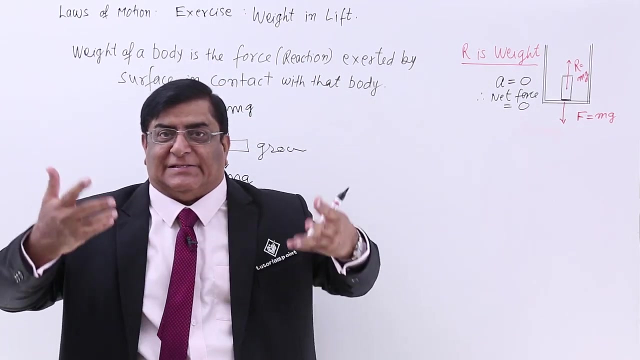 If I am pressing the ground. the ground is pressing my body upward. With how much force? mg. Now I feel an action on my feet. Somebody is pressing it. A surface is pressing it. With how much force? mg. Like somebody is pressing me here. Somebody is pressing me here. Something is pressing my foot upward with certain force. So I have an experience. I have a feeling that somebody is pressing. 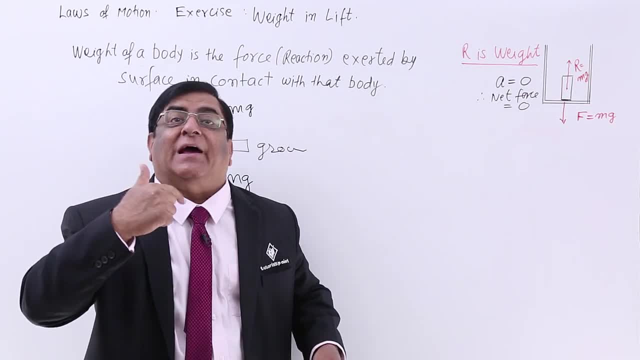 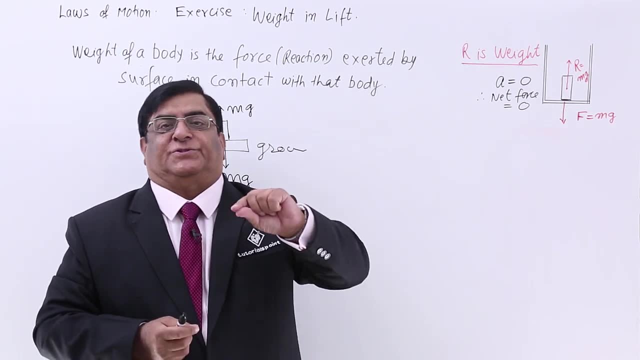 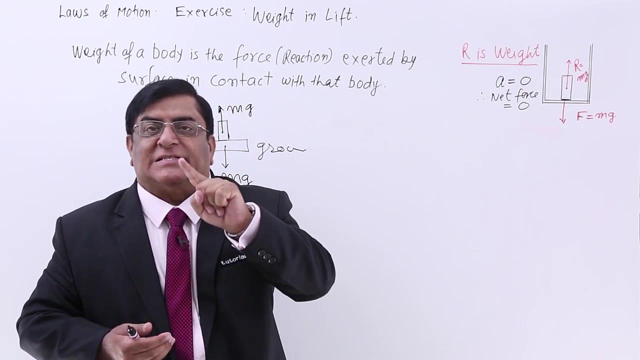 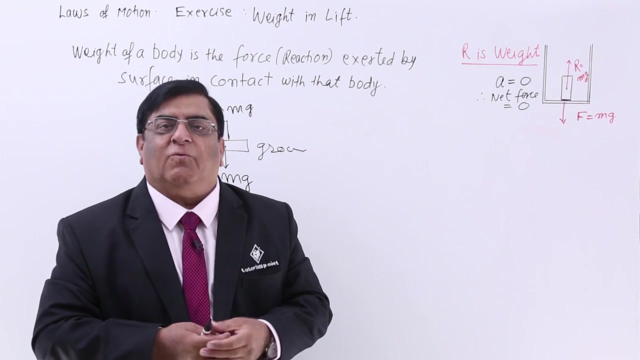 That feeling, that experiences, is my weight. Yes, So weight is an experience of force which a surface in contact is applying on me. If earth does not apply this force, then I say I am weightless. It happens when we fall from, say, aeroplane. 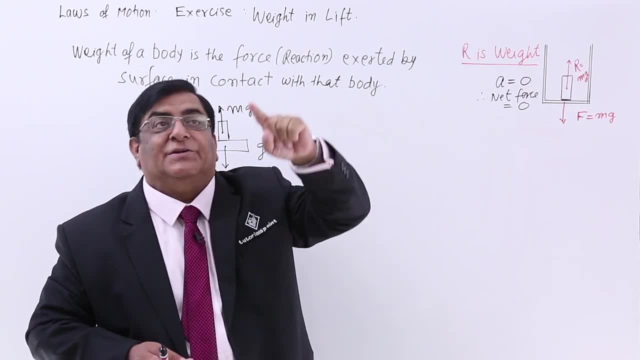 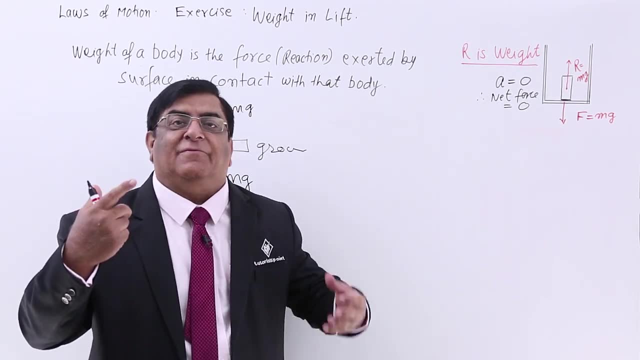 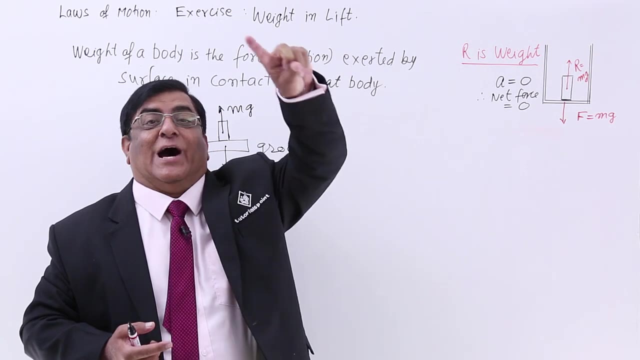 from a high mejoneer to a manyjoneer building. at that time, during the fall, earth is not pressing my feet because it is not in contact. at that time I have a different type of feeling. you have that feeling when, when you are coming from that that large thing, what you call it, at that time you have a sort 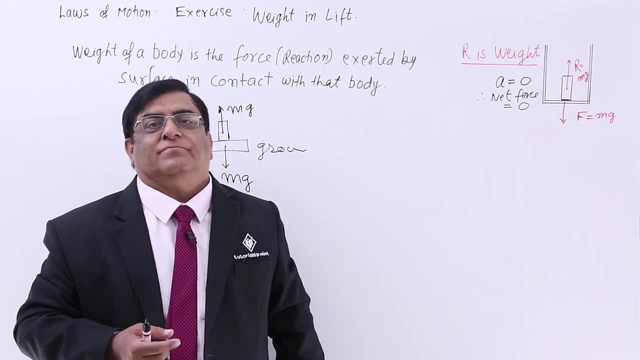 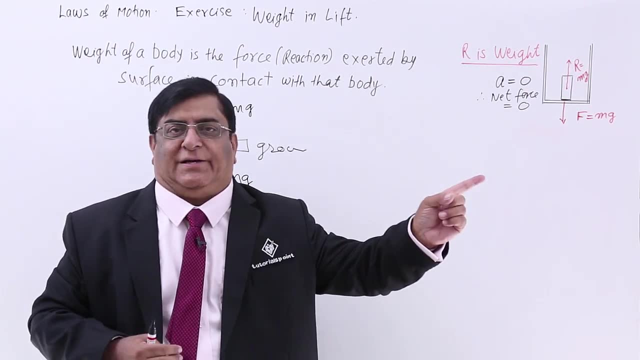 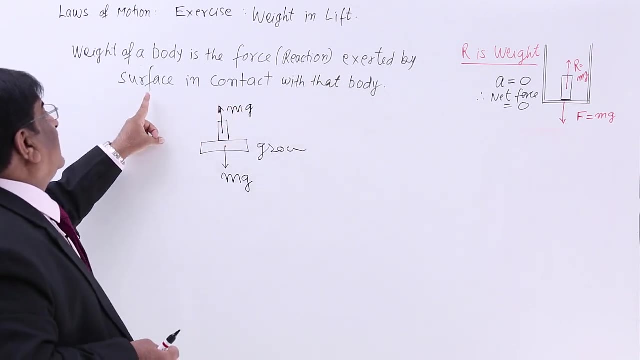 of feeling when you are coming down, that is the feeling of no weight, because at that time earth is not pressing. you will come to that. but first, what is weight? weight of a body is the force of reaction exerted by surface in contact with that body. so this is surface. 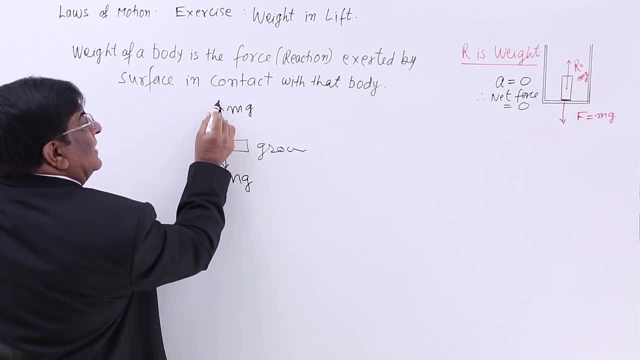 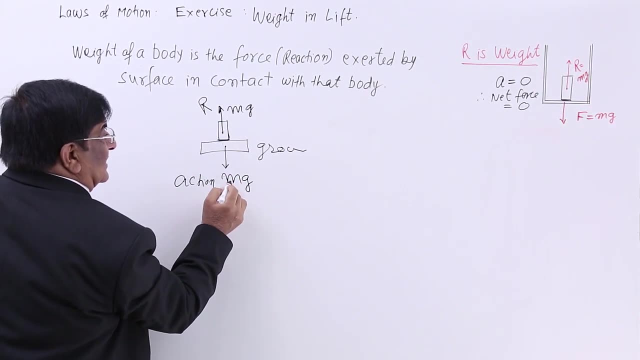 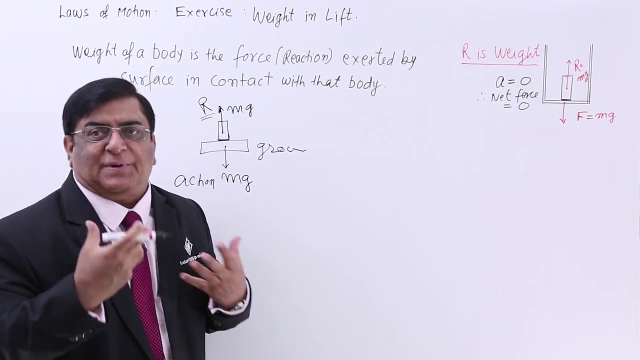 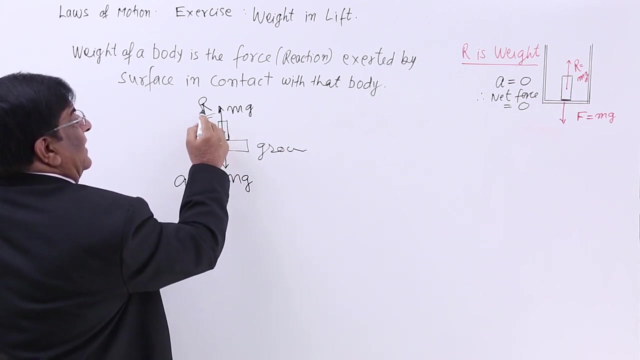 in contact with this body. it is pressing this body with reaction, because this body is having here action. this is action, this is reaction, and this force of reaction gives me a feeling of an experience. that feeling is known as my weight. this is my weight reaction. okay now, 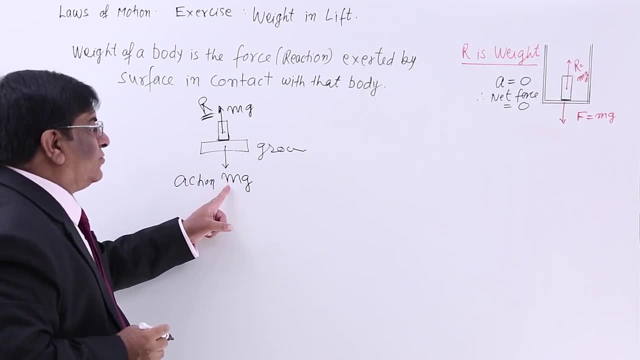 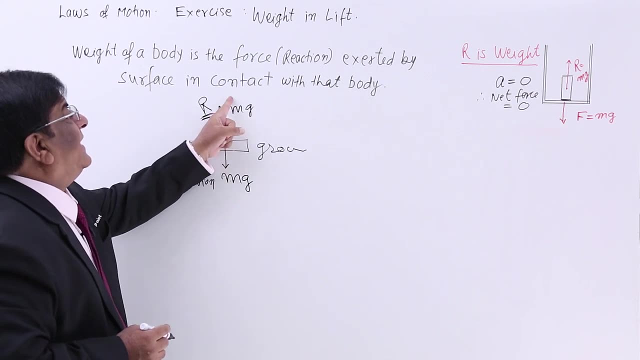 my action on this is mg. according to the role, action is equal to reaction, so the reaction is also mg. therefore, I say my weight is mg, so my weight is not the force exerted here. my weight is the reaction Exerted by this body on my body. if there is a change in the reaction in spite of this, 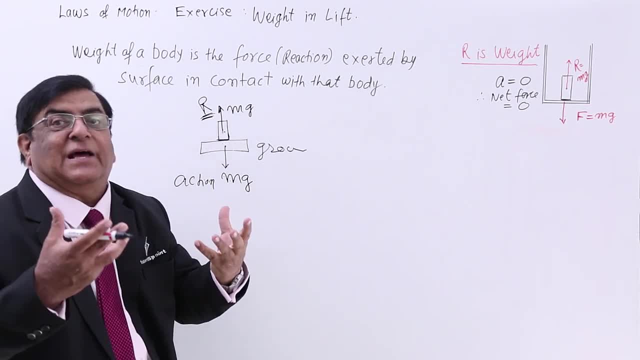 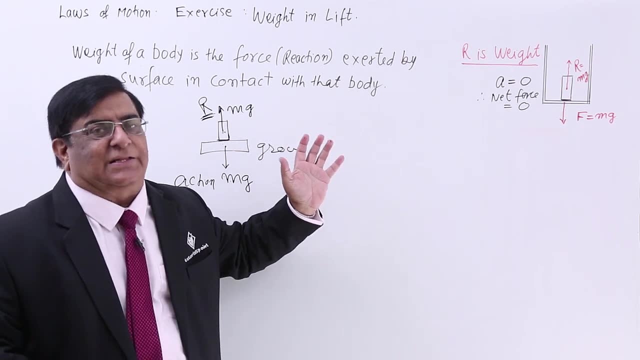 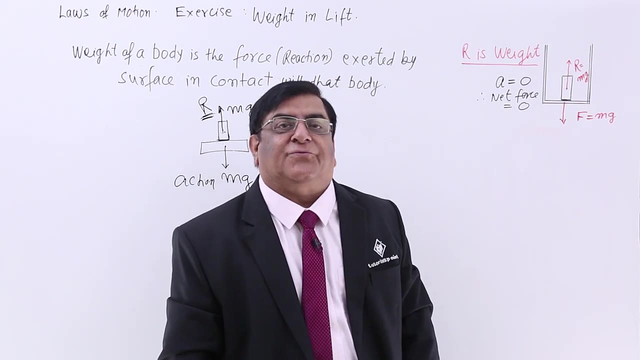 if there is a change, then I will experience that my weight is less. yes, that happens, and with help of this, by understanding this principle, now we are in a position to find out our weight in a different frame. we have seen the meaning of frame of reference. 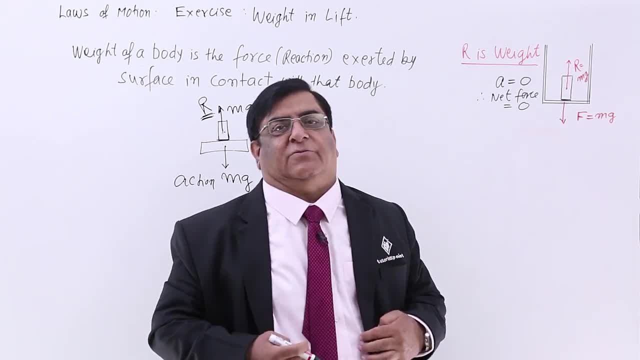 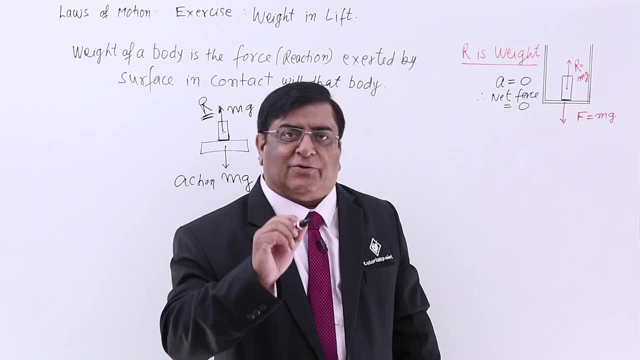 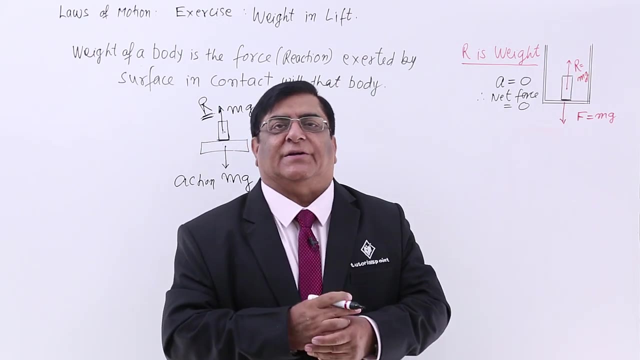 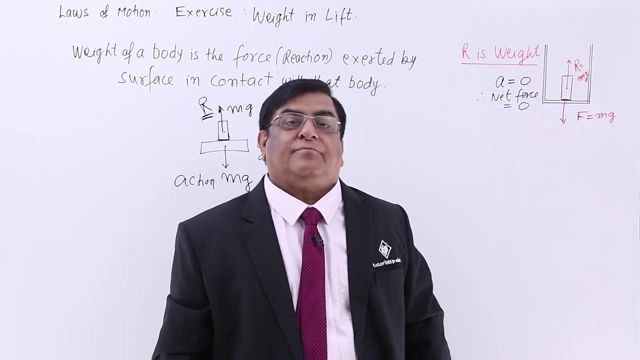 So If frame in which we do the calculation if it has no acceleration, then we calculate the things in one manner, and if that frame is having its own acceleration, then our calculations change. and here we have that type of frame. now we want to do the calculations in this. 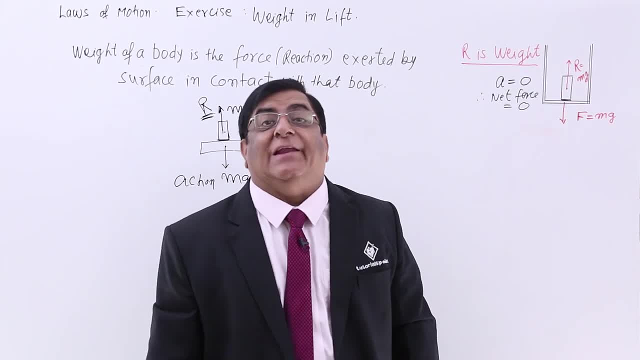 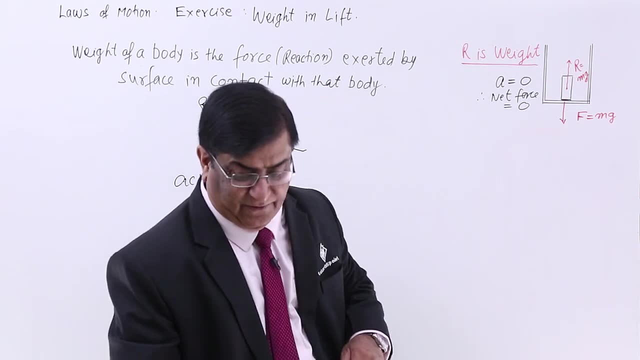 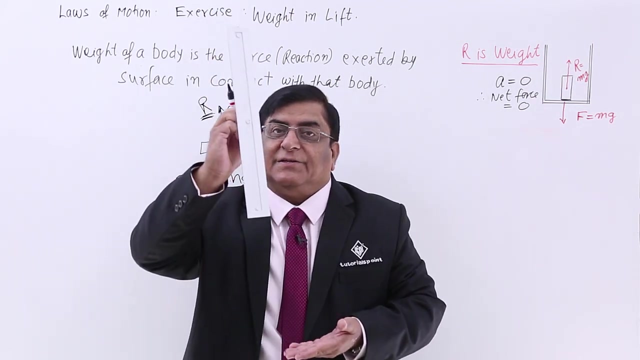 frame and we call this frame as lift. Yes, Yes, Yes, elevator. So in this lift, what is the specialty of the lift? It is at velocity 0 and then it accelerate and reach a particular velocity. Say, here velocity is 0, this velocity is 1,. 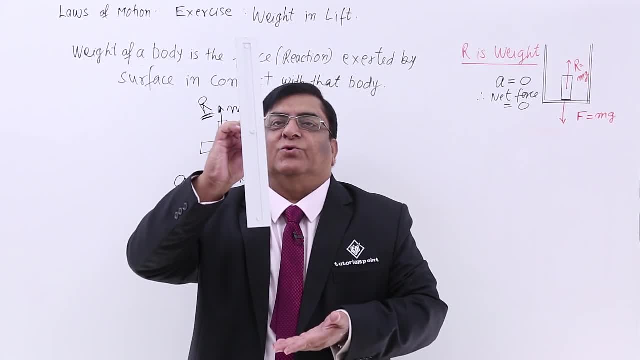 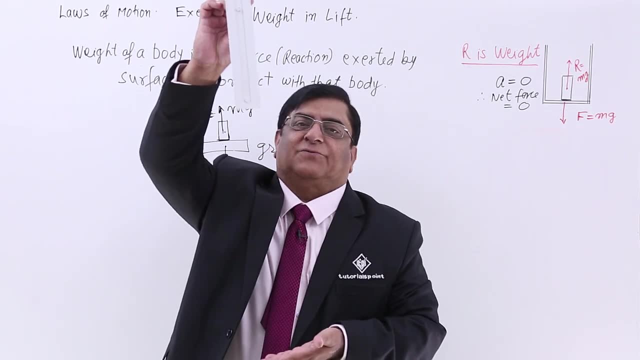 2, 3,, 4, 5.. Then it goes at the speed of 5, 5, 5 and then it becomes 4, 3, 2, 1, 0.. Go to the next floor again lifts up. initially there is a acceleration. that acceleration: 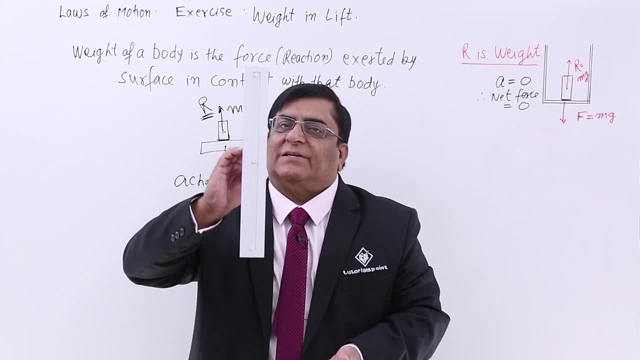 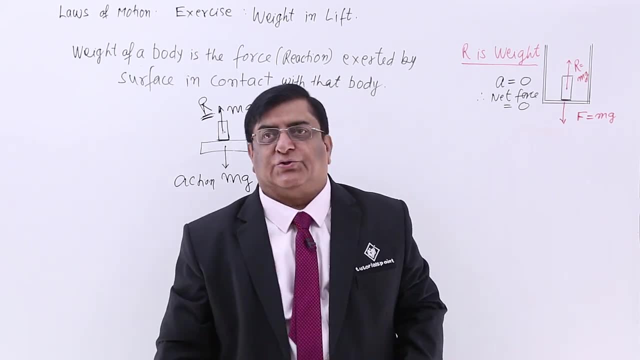 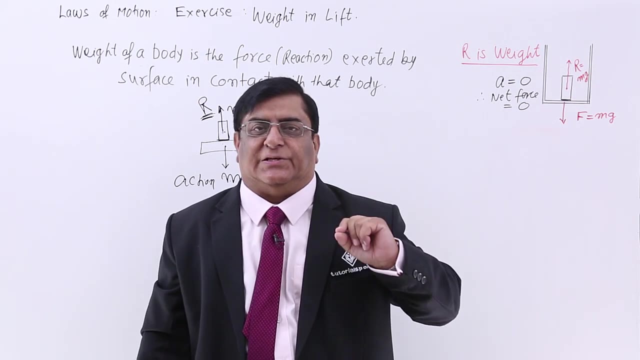 increase its velocity, then it goes by certain uniform velocity and then there is a retardation again it comes to stop. So we are talking about three stages. One lift is at rest. the acceleration is 0. it is the same state when the lift is having. 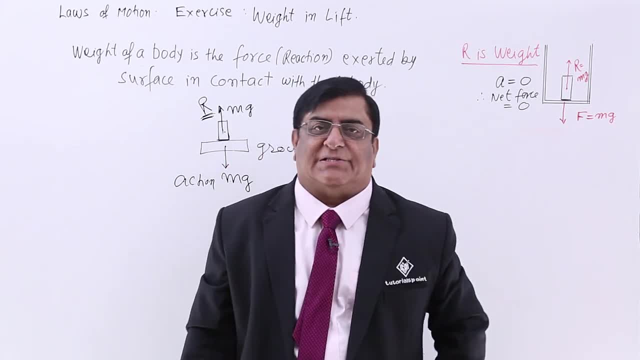 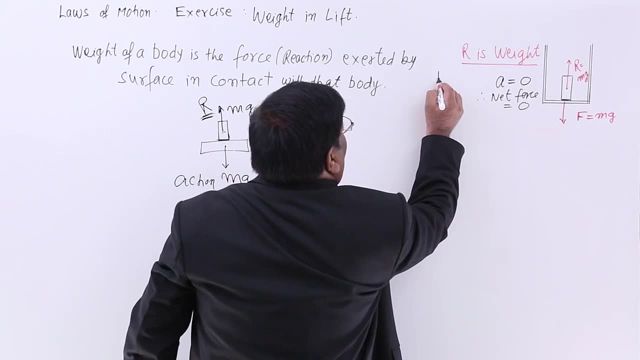 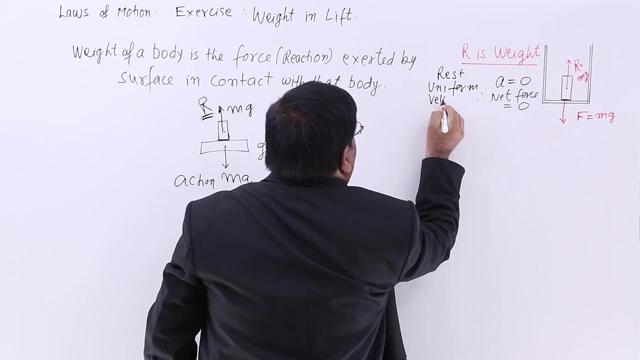 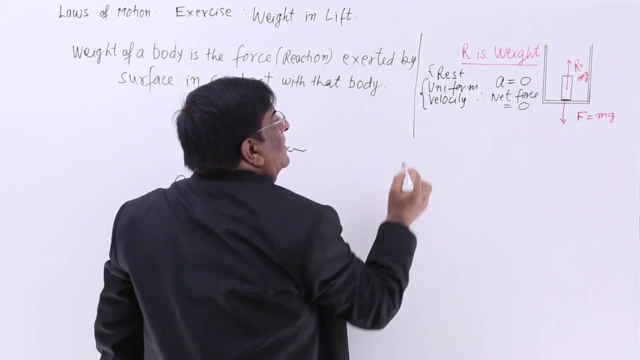 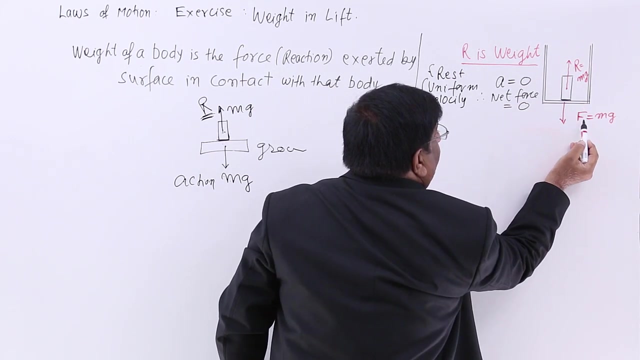 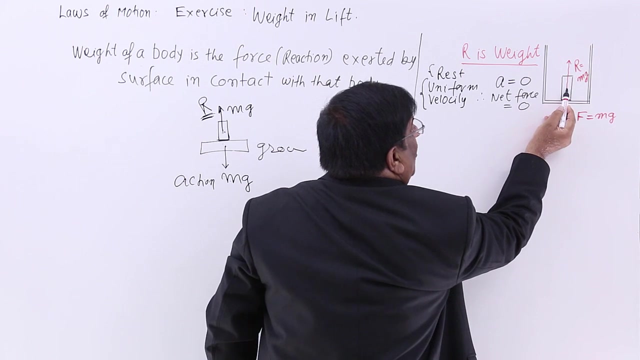 uniform velocity. at that time also, acceleration is zero. Now, when that thing is there, acceleration is zero. it may be at rest or it may be at uniform velocity. Both things is possible: rest or uniform velocity. Okay, in this case, this body is pressing the floor of the lift with a force mg As a reaction. this floor is pressing the body of person with the same force mg and what we call it reaction. 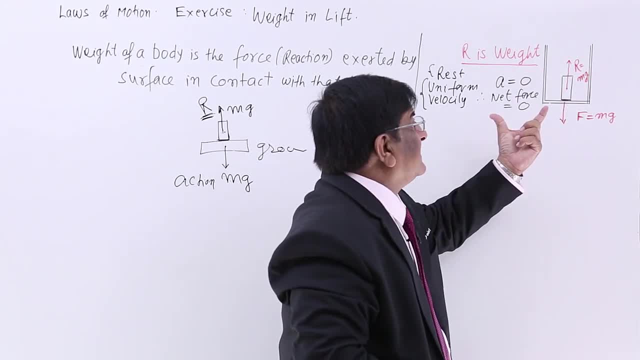 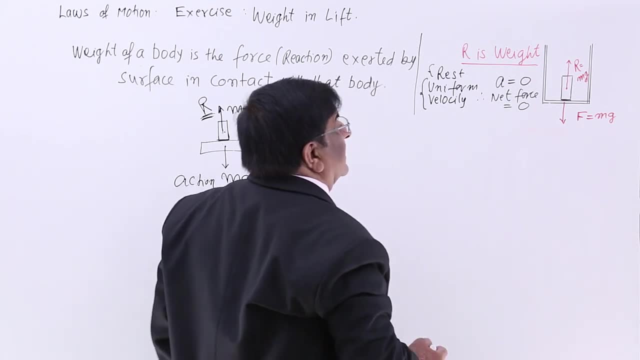 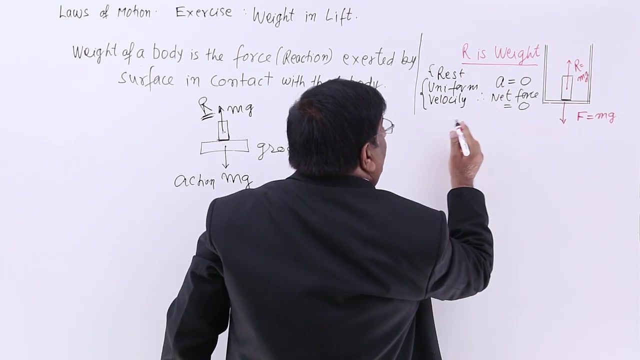 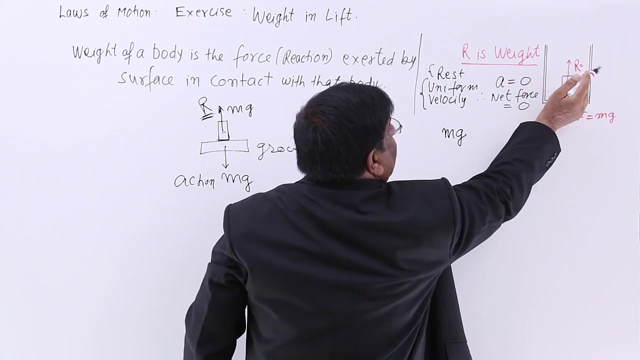 So reaction here is mg. As a result, what is the net acceleration of this body? This is not moving, so net acceleration is zero. If I make a free body diagram here for this body, what is the net force? The force acting downward is mg. The force acting upward is reaction R. 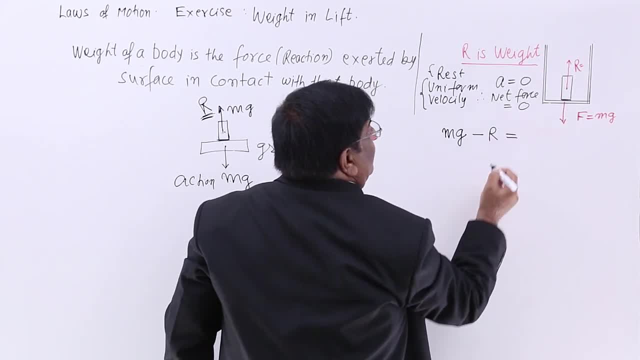 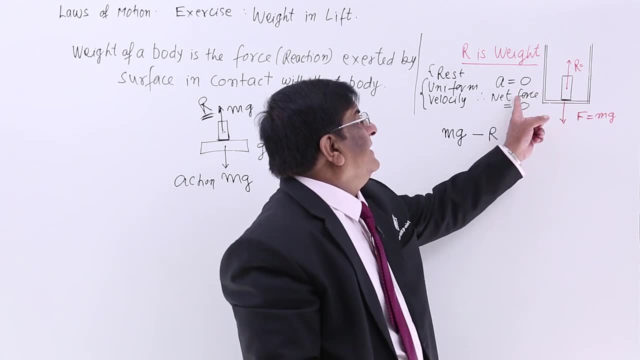 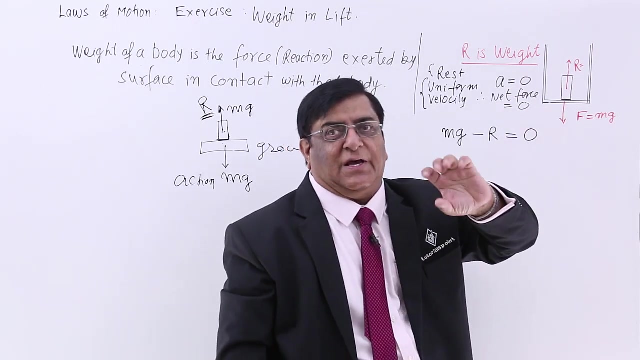 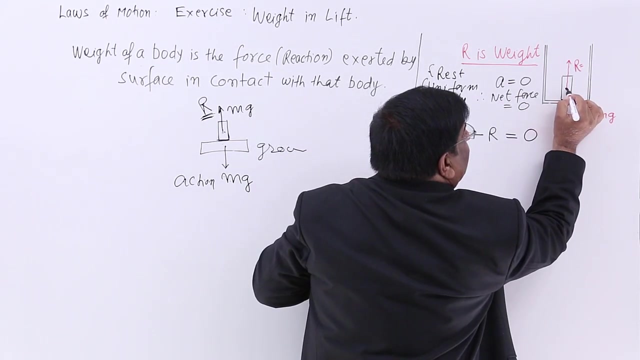 And what is the resultant? acceleration: Zero. Acceleration is zero. so what is the net force on this body? Zero. So on this body there are, you will say how net force. Okay, Here this body is being attracted by the earth. With how much force? mg. 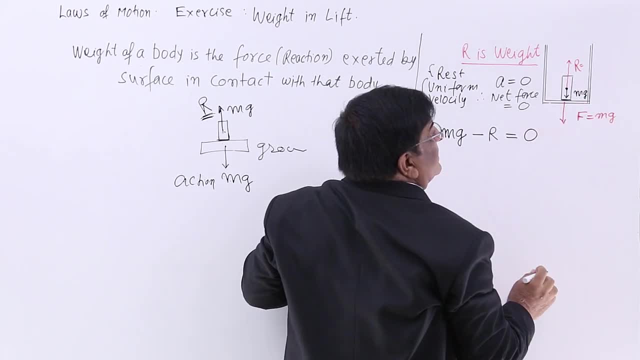 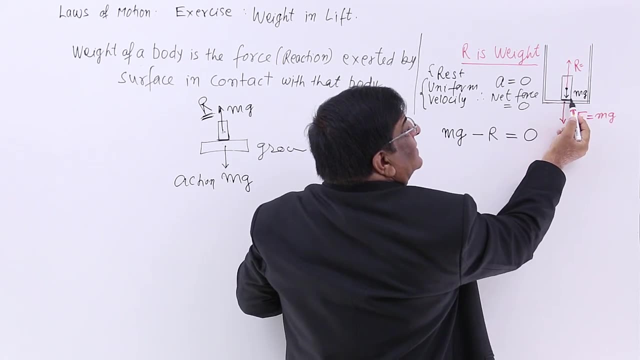 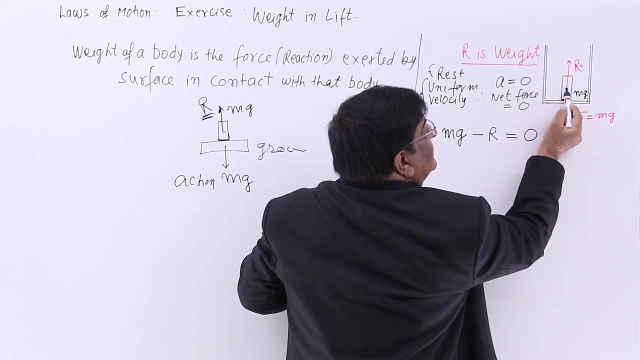 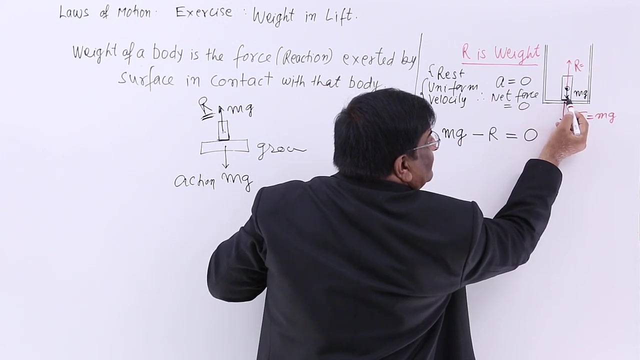 It is pressing the floor with the force mg because there is no motion. So all this force mg is transferred here And this floor in turn making the force mg Okay, Okay a reaction. So what we find here on this body, Mg acts downward, reaction acts upward. that 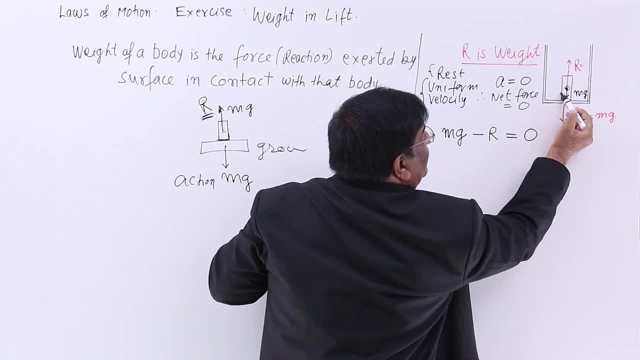 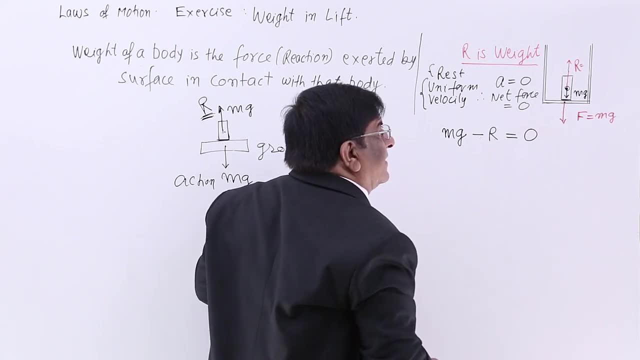 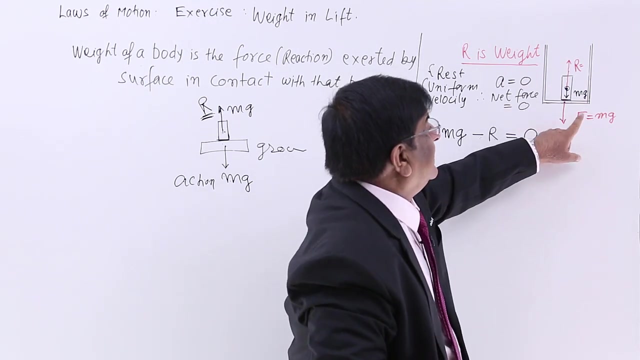 is negative Mg minus R. and what is the net force here? Answer: net force is 0 because body is not moving. So this is net force Again. this Mg is what This Mg or this Mg Earlier students failed to understand. They think that this is the Mg, this No, because 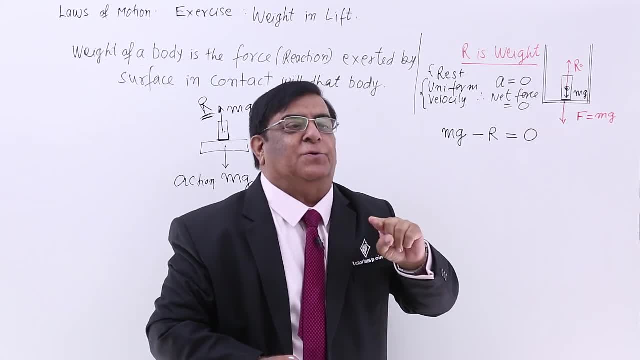 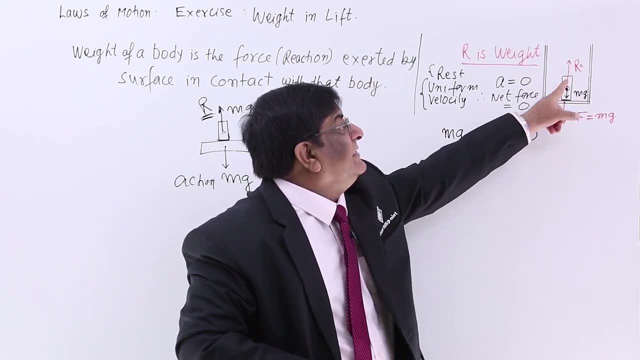 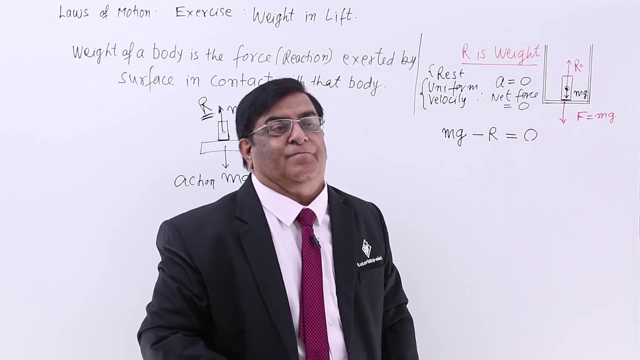 the rule of addition of vectors are: all the vectors should be acting on one body, then you can add them. One vector which is acting on the lift, this vector which is acting on the body cannot be added together, cannot be subtracted. So if we want to do an addition, 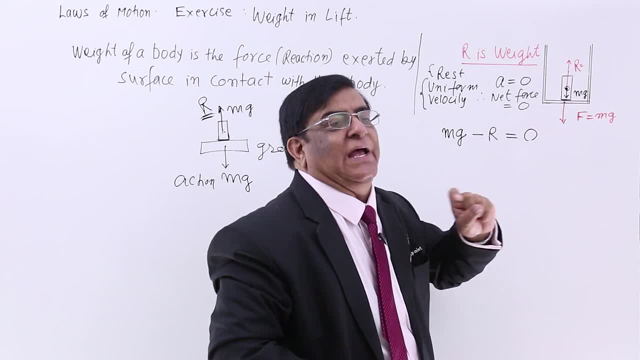 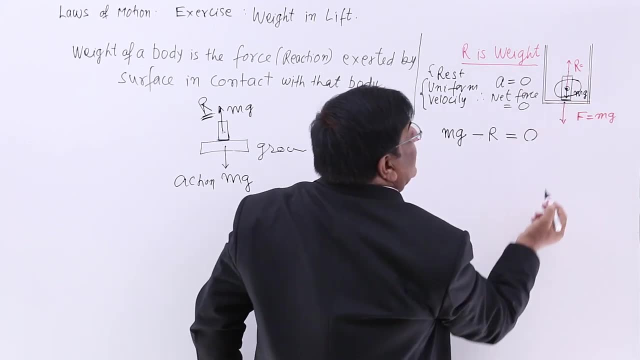 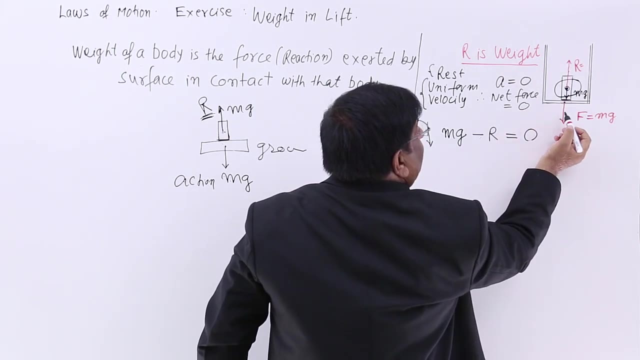 equation we have to find R: All the forces acting on a single body, rather on a single point. So this is the point I am taking Here: earth is pulling it down with Mg. The reaction is by what? Reaction is by the floor. Why the force has to, why the floor has to give a reaction? Because 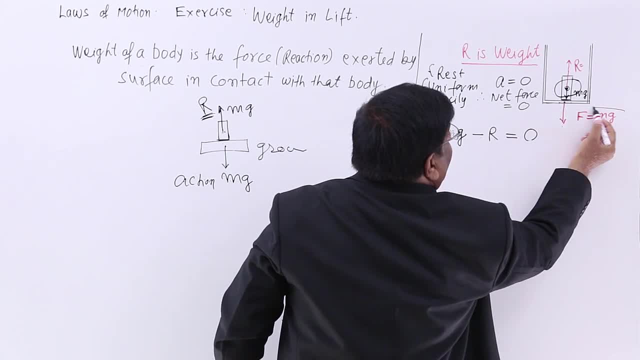 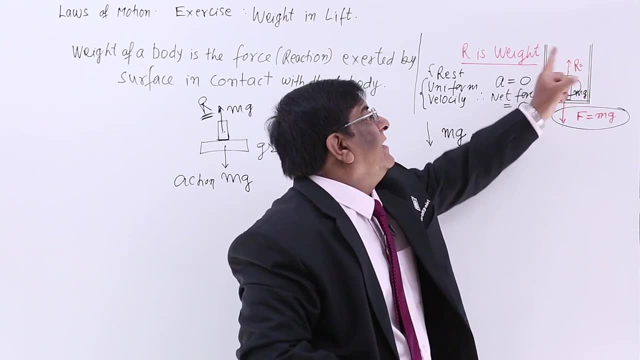 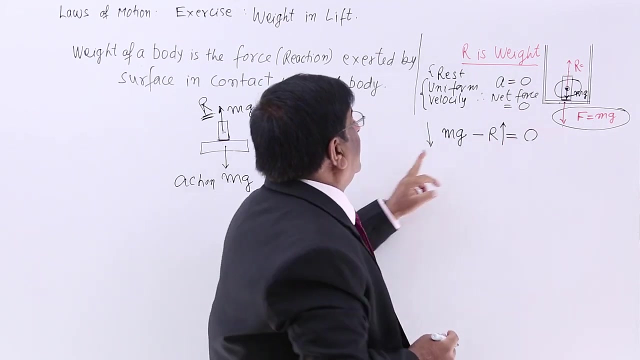 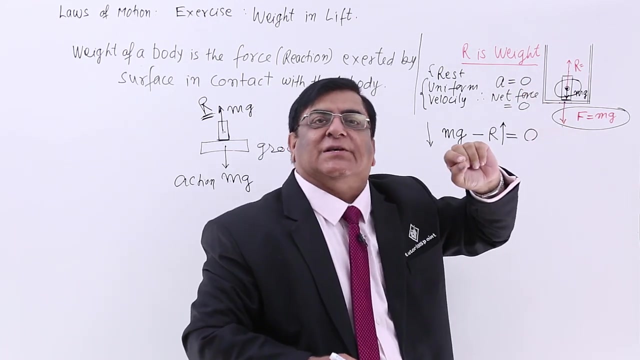 the floor is being pressed by force Mg. This is the reason why it should give a reaction. So it is giving a reaction in upward direction. Now this is the total, because one is downward and one is upward. This is the net force and we find acceleration is 0. That proves that net force is M into a that is 0, 0.. So you, 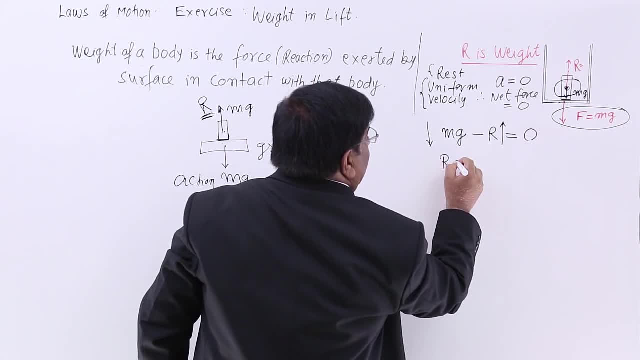 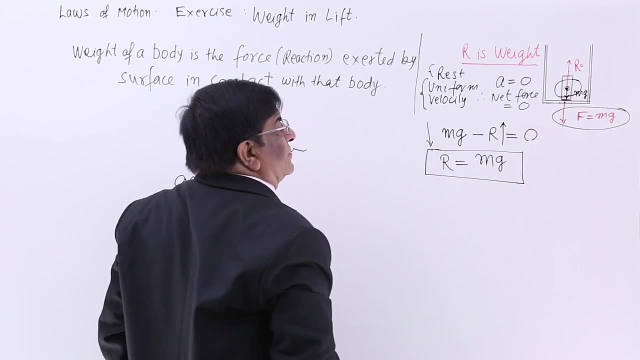 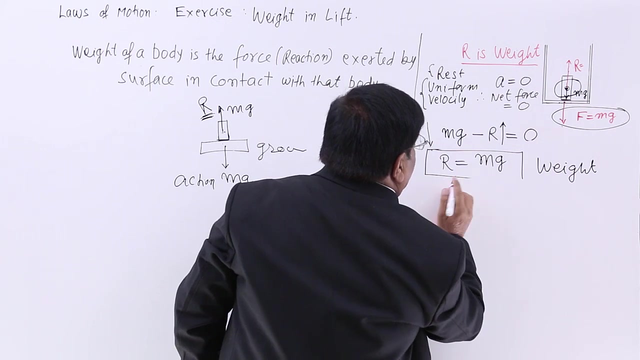 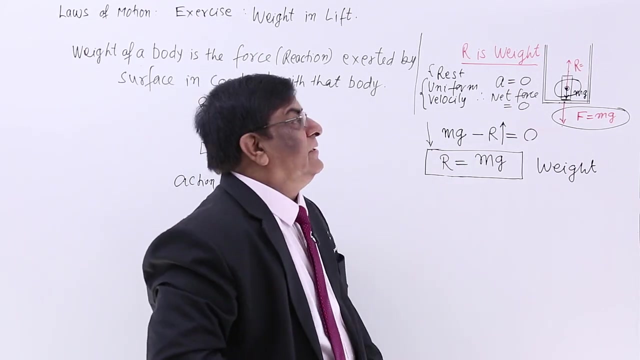 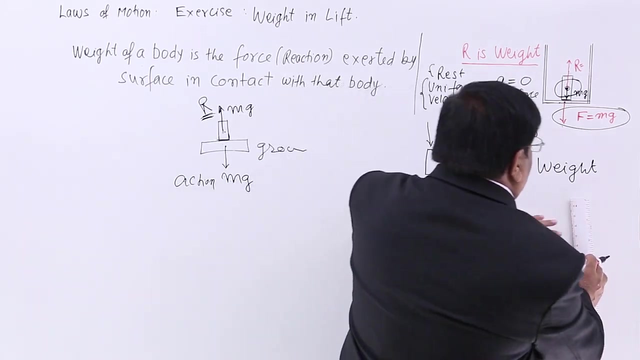 transfer it. on this side, R is equal to R is equal to Mg, R is equal to Mg and reaction is what Reaction is weight. So weight of the body is Mg. Okay, In this case, very simple case. Now we go for the second case. In second case, the lift. 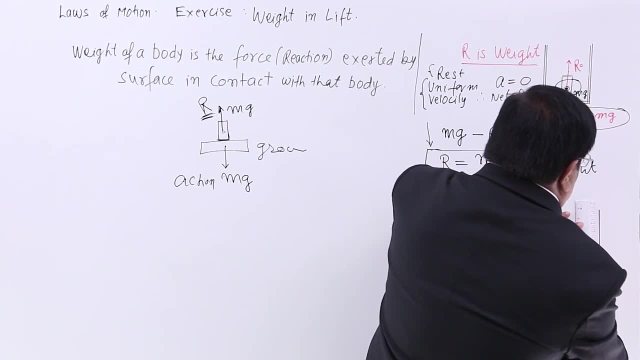 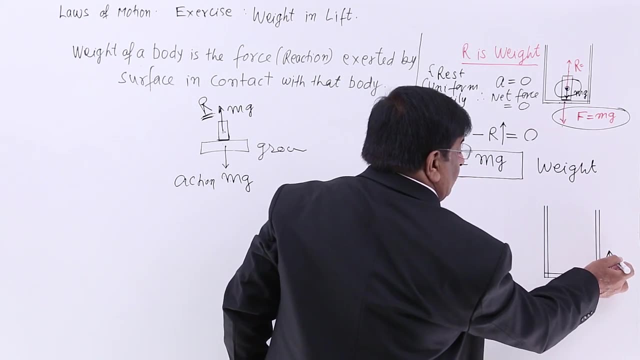 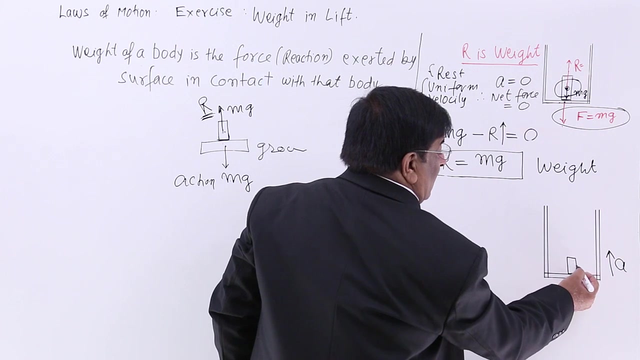 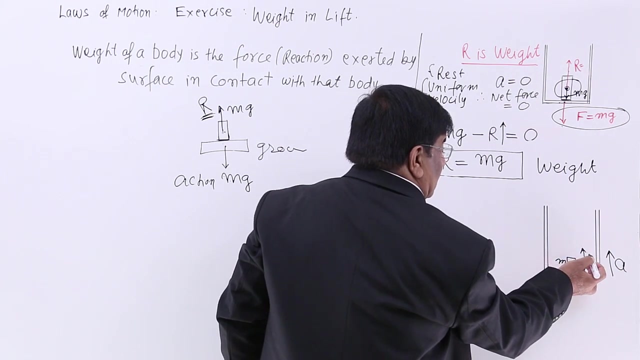 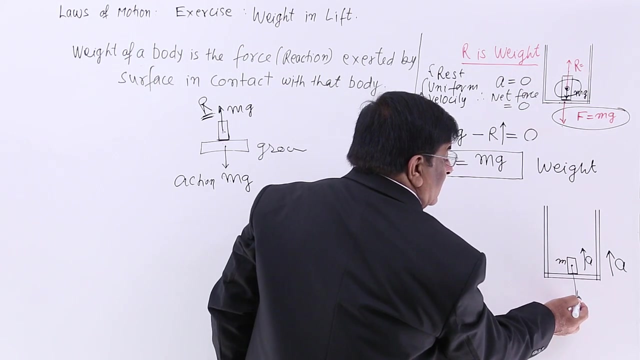 is moving up with certain acceleration. This lift is moving up with a net acceleration a, And here is a person in the lift having mass M. So if the lift is moving up with the acceleration, this person is also having acceleration a. Now this person is being pulled down by the earth with a force equal to r. This is 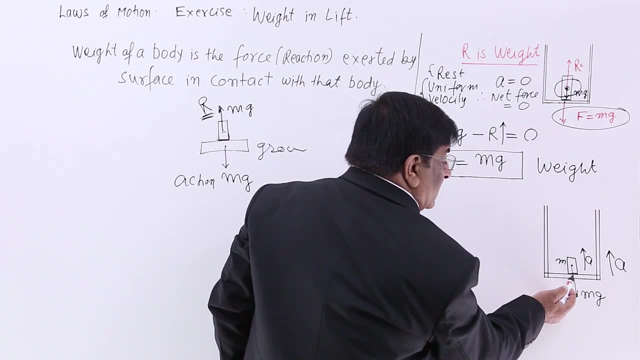 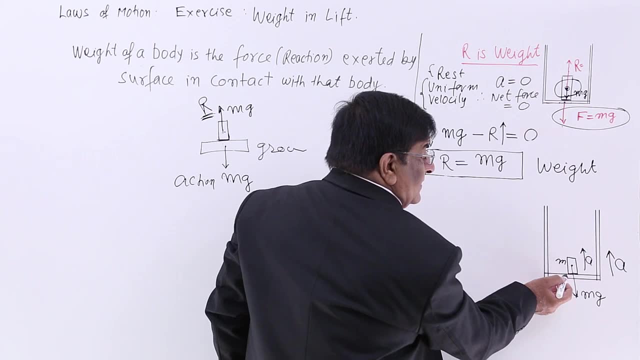 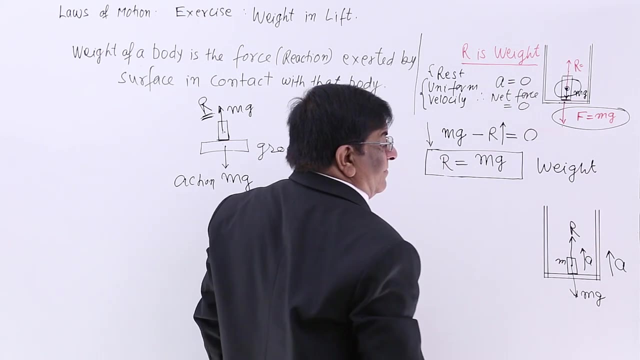 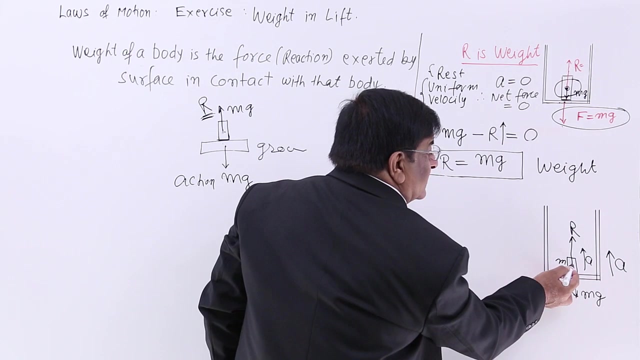 mg, because it cannot cross this. this compress the floor and in reaction to that compression, this floor is pressing this body. upward reaction, reaction by the floor. So on this body, when we talk, there is a force of gravitation. downward there is a force. 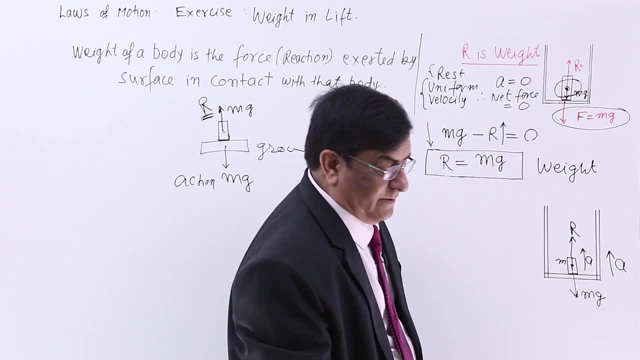 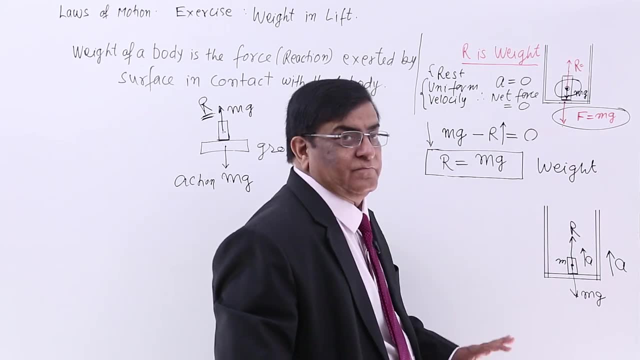 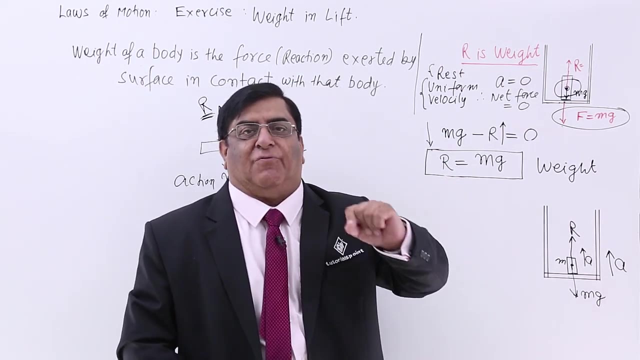 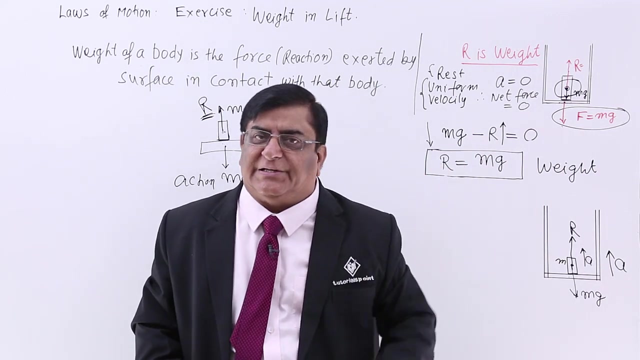 of reaction upward and, as a result, the body is going up. that is, the total system is going up. that is the net force, because unbalanced force, net force- is the one which is responsible for motion and it is moving up. So that is the net force. how do we calculate the net force? the balance force? sorry, unbalanced. 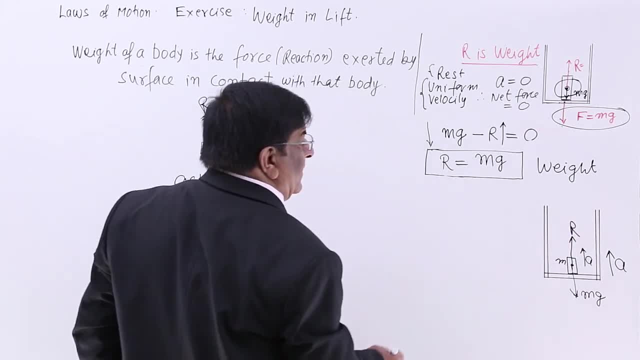 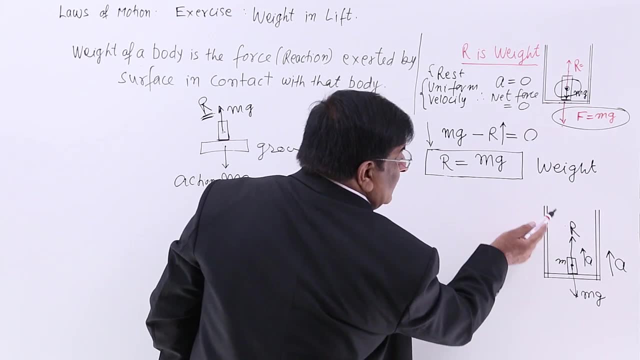 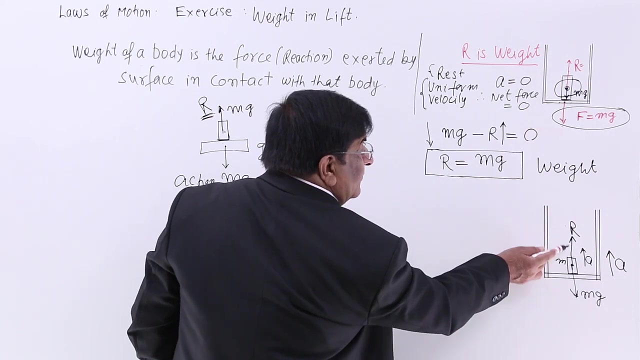 force. So make the total of the forces here: is the R greater or Mg greater? answer: because it is going up. that shows R is larger than Mg. If Mg is larger it will come down. if R is larger it will go up. and given condition to: 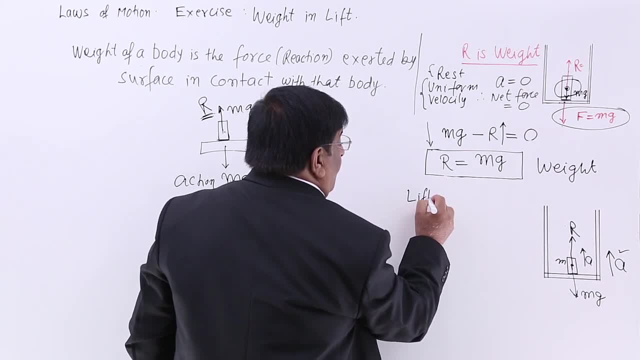 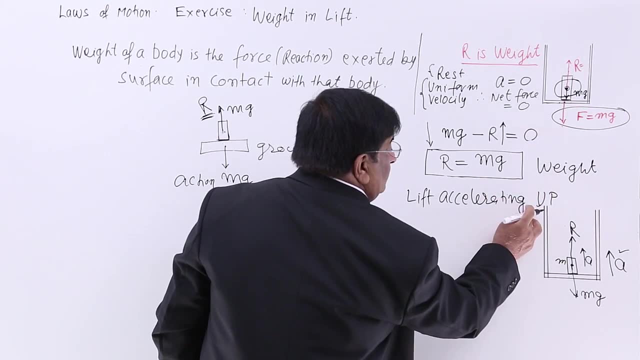 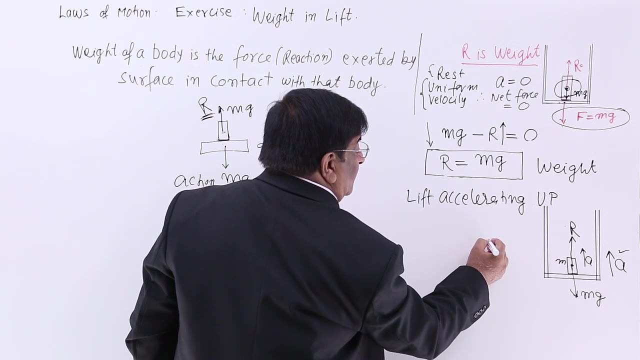 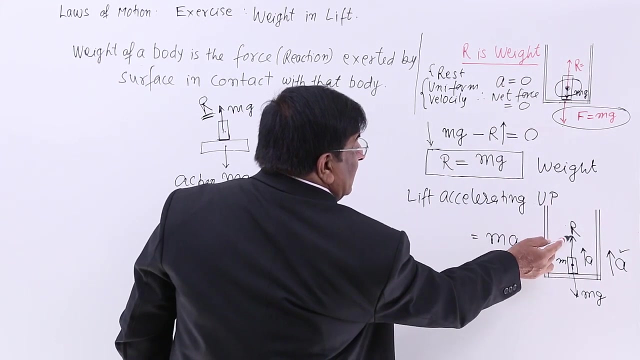 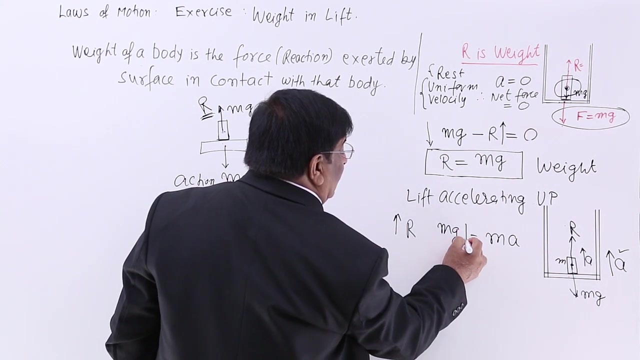 us is that lift is moving up, Lift accelerating up. Okay, Lift is accelerating up. Now, if lift is accelerating up, how much is the net force, Ma? How do we get this calculation answer: R is force acting up and Mg is force acting down. 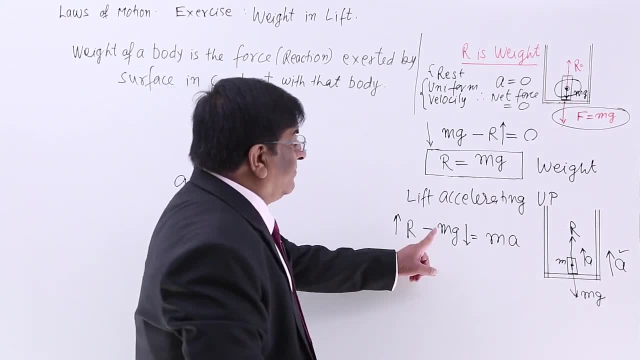 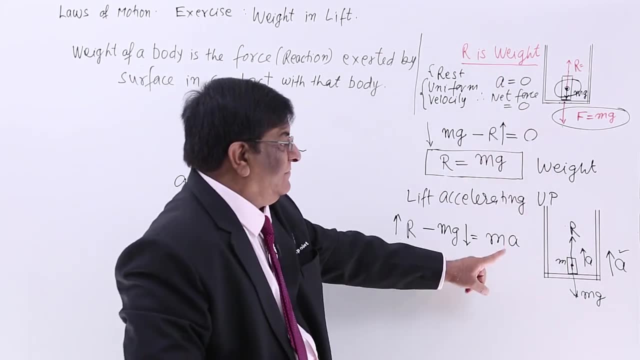 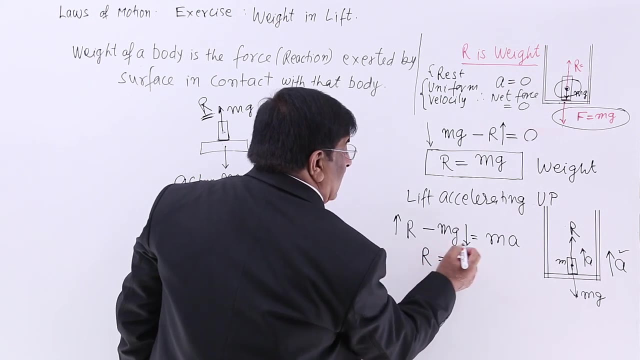 So it should be minus. this is the net force: up minus down. get the resultant and because of this resultant it is going up. up is our positive direction. This now, with this equation, R is equal to this will go here and M is common, we find 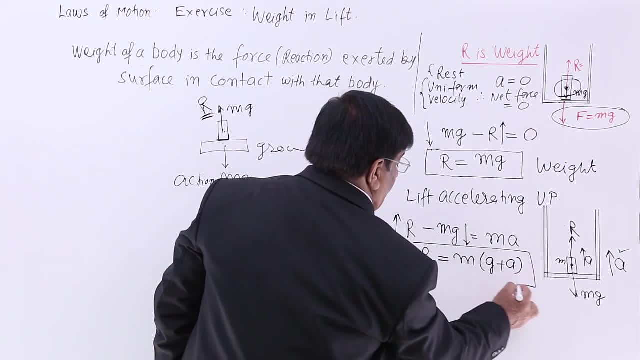 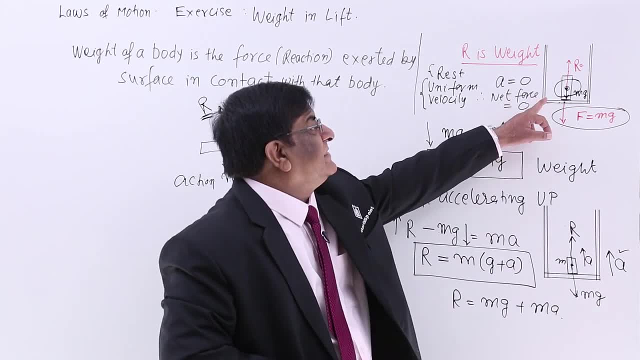 So this is the net force. So this is Mg plus Ma. SO this is the net force. So this is the net force. So you know, the net force is not there, but the net force is there. So I say m 22, O, Ma and g Nicolai. So if this now this means J meet 0. 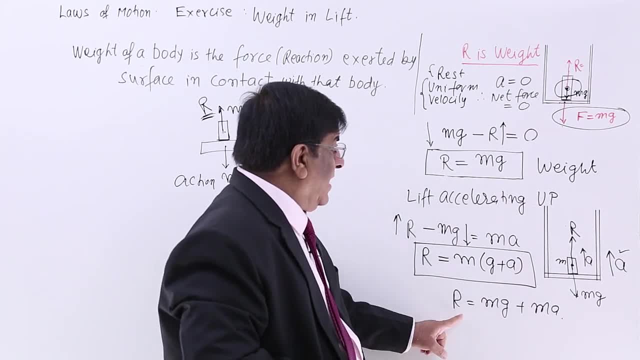 Then my difficult reflection here is: that is the net force. The net force is the same, that is, a basiccticamente nonlinear Mg plus A square equal to the correct expansion weak pair. Now, when it was stationary, how much was the reaction MG? That was our weight. now, when it is moving up, how much is the reaction Mg plus Ma, which? 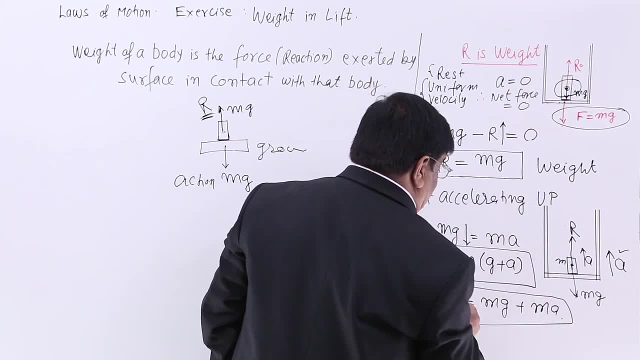 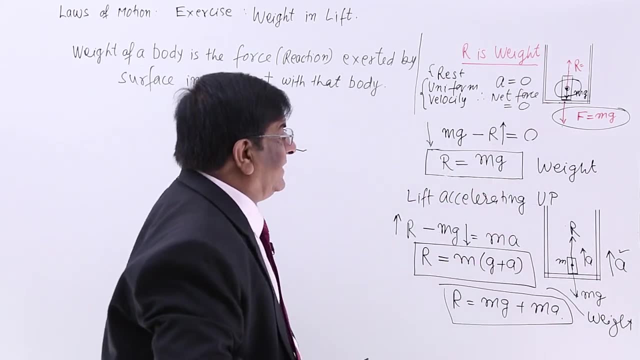 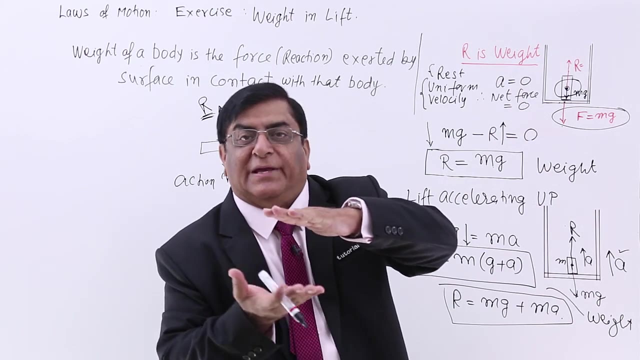 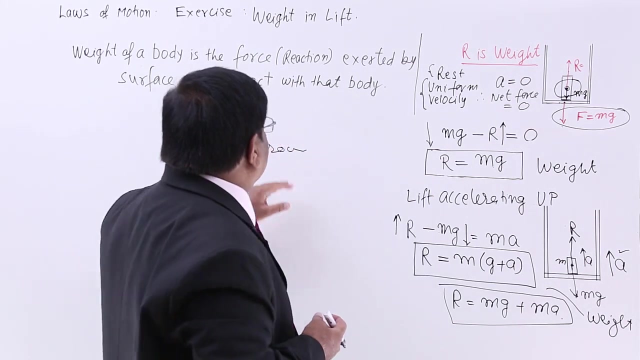 is more than Mg And this is our weight. So what happens to weight? has it increased or decreased? Answer is: it has increased. So our weight increase When, when we are being출 soap pushed by certain force, as in this case, But when we fall down, there is acceleration downward. 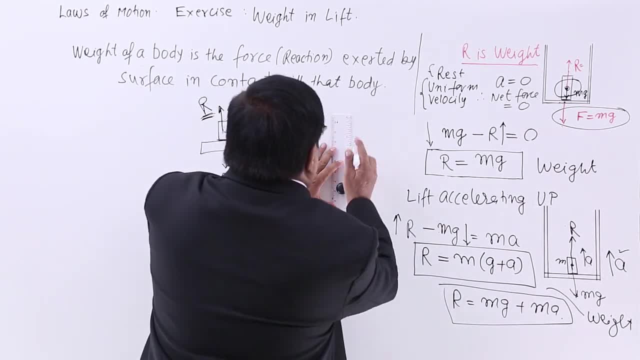 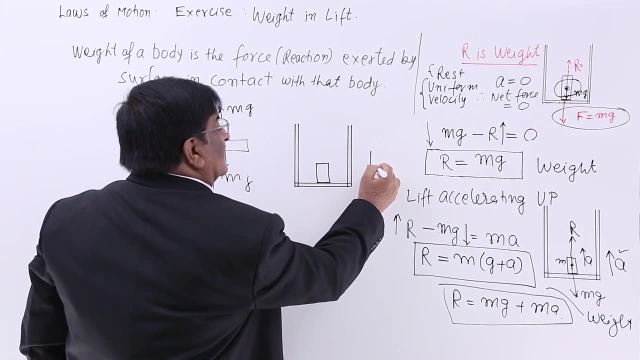 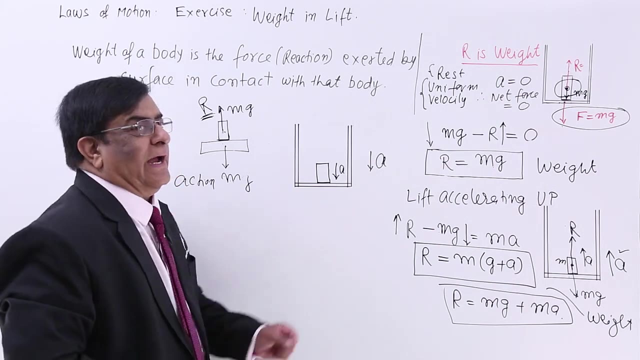 and for downward acceleration. we make a situation here. Here is the person and the lift is coming down with certain acceleration a. That means this person is also coming down with acceleration a. and where there is an acceleration, there is mass. That means there is an additional. 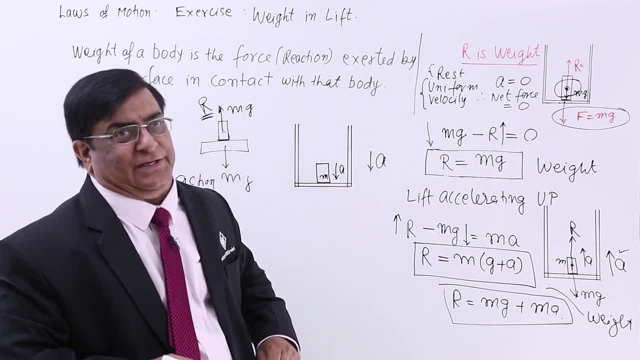 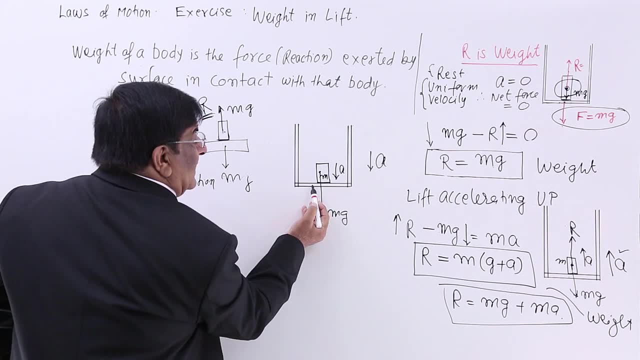 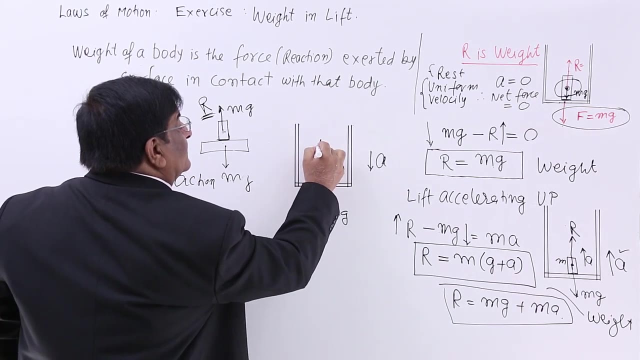 force on this person m into a in downward direction. Again, earth is having a force mg on this body and this surface does not allow it to puncture. That means it is having a reaction on it- upward reaction. The force mg on this person is m. 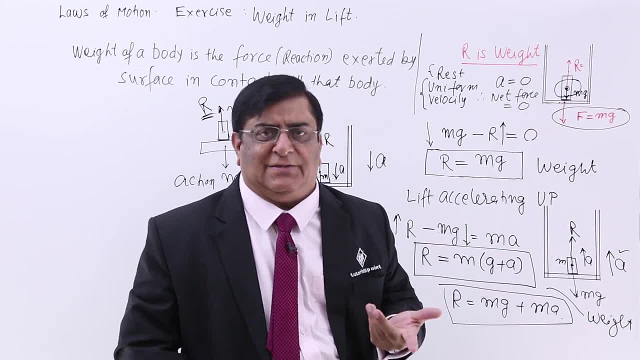 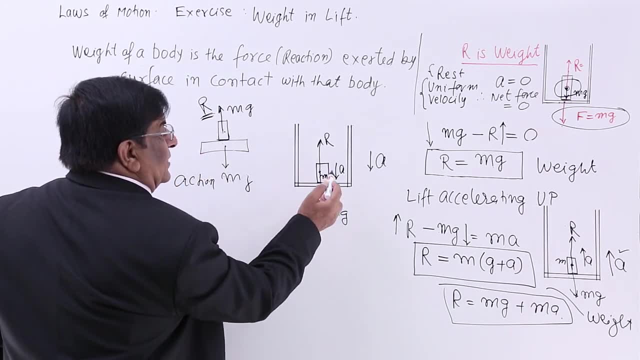 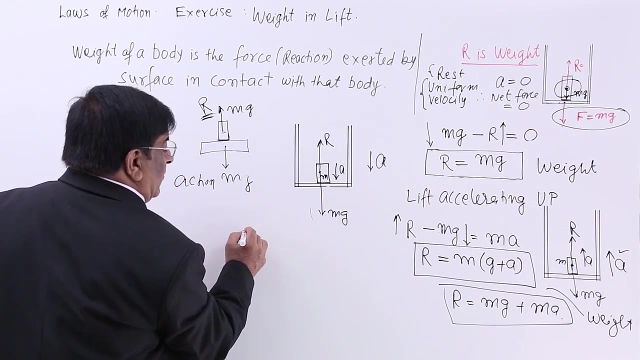 the surface. we are not showing it because we do not need it. We need only force on one body, and that one body is inside. So here, which one is larger? Because the final force, the net force, is downward, we assume that this must be larger. So the equation will: 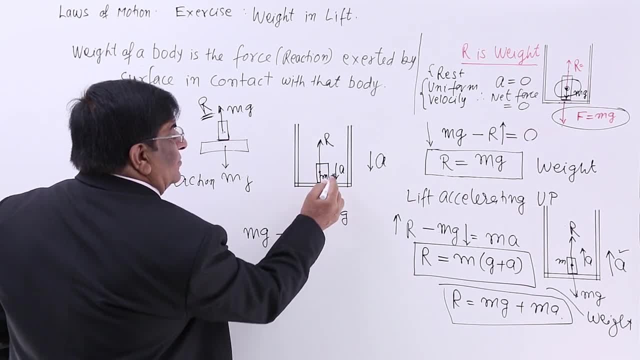 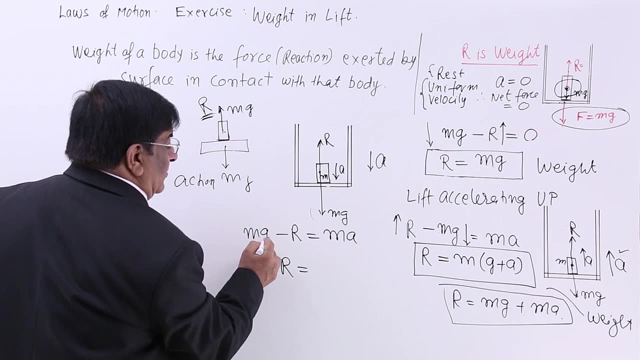 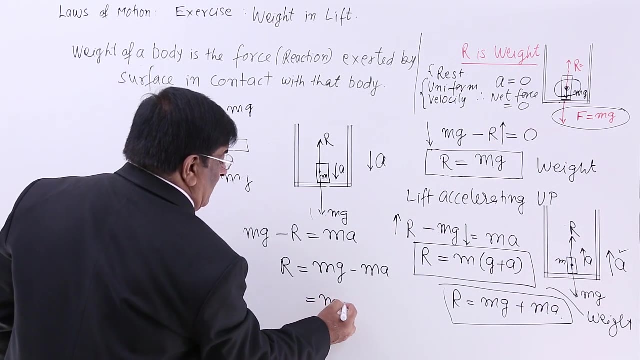 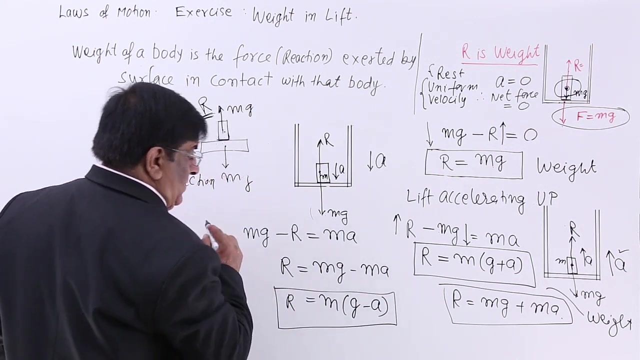 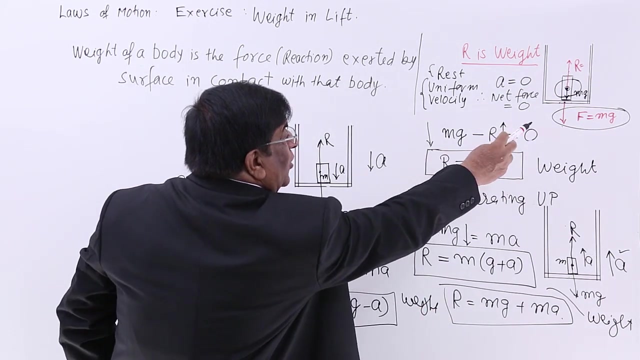 be Mg minus R, which is equal to resultant force, that is Ma. So how much is R equal to? R is equal to Mg minus Ma. Mg minus Ma, That is Mg minus A. This is reaction and this is weight. Now, at rest, weight was Mg. When it is coming down, it is Mg minus something. 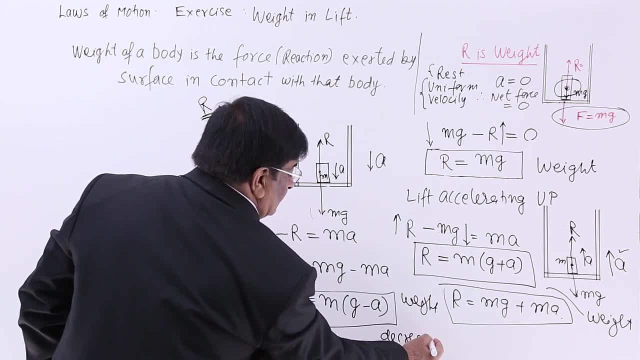 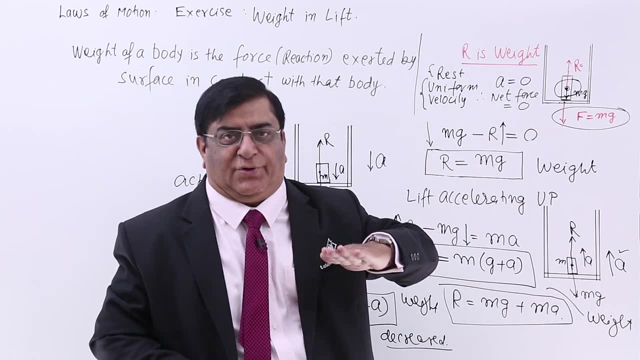 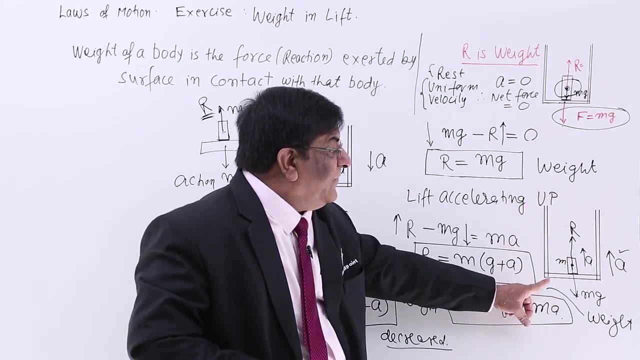 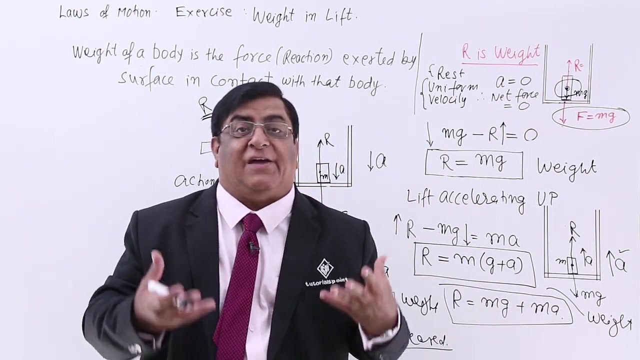 That means weight has decreased. So these are our result. When the lift is at rest, we experience our natural weight, Mg, which is the weight on the ground. When the lift is accelerating up, we feel additional weight- How much is the addition, Ma? and we feel that we have become heavier At that. 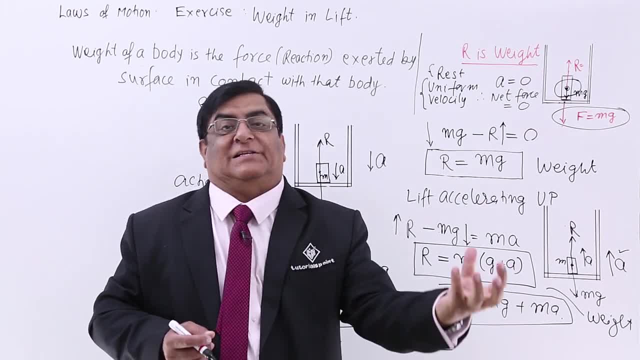 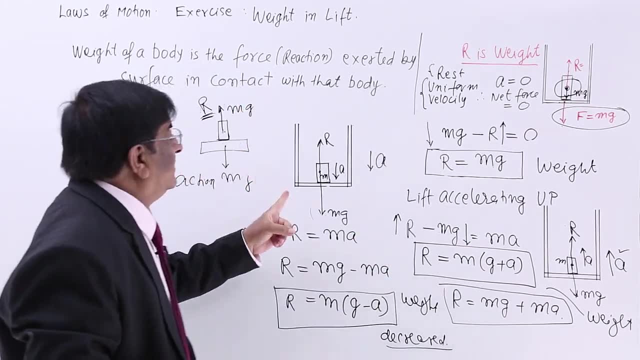 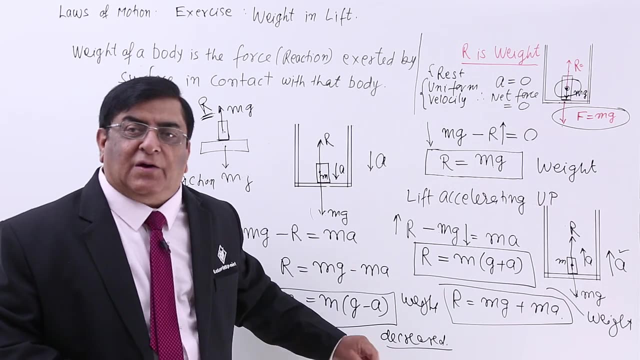 time. if you want to lift your hand, you will find it is difficult because it has become heavier. Every part has become heavy when we are accelerating up. Contrary to that, when we are accelerating down, we feel very lightweight. It is decreased. 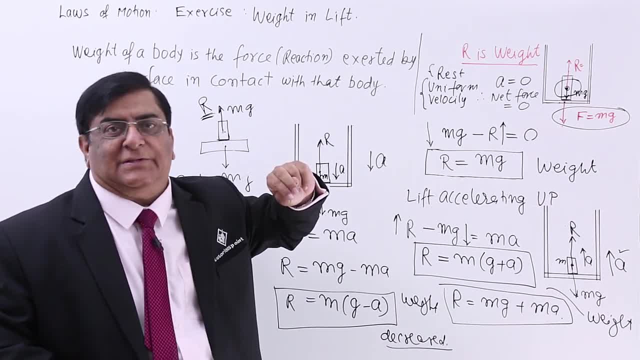 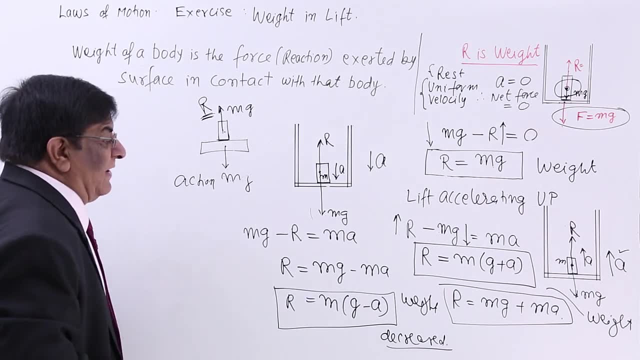 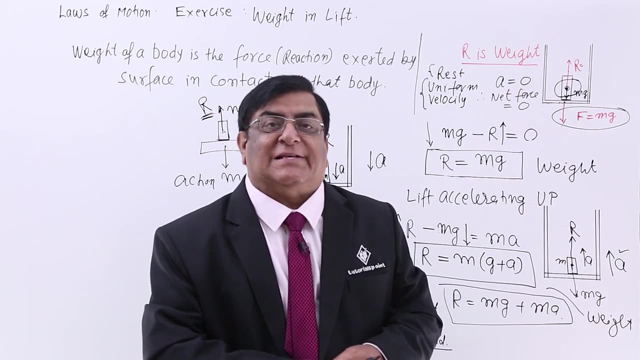 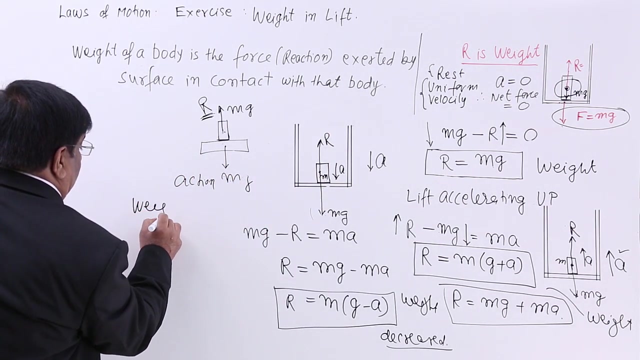 Now, when we jump from the aeroplane, then our acceleration- this acceleration is equal to G. Then what will happen? The reaction will become zero. That weight will become zero. That is known as condition of Weightlessness- The weightlessness- and that body is known as free-falling body. 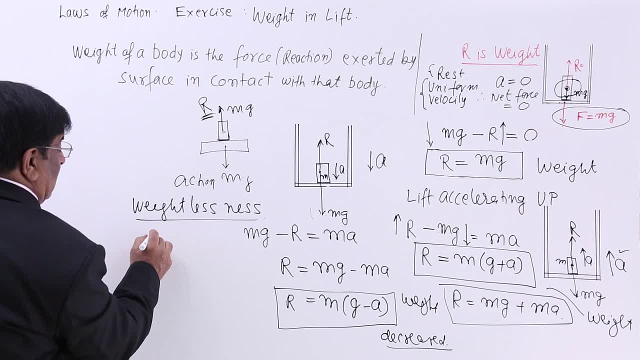 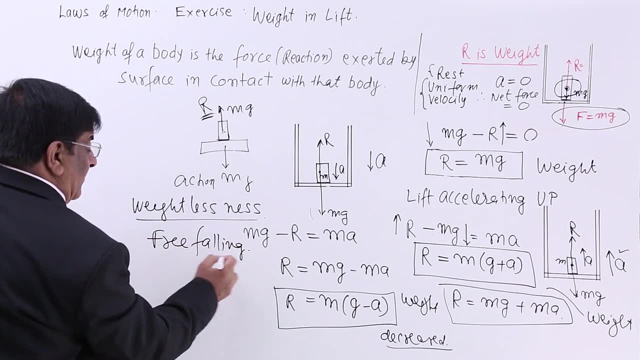 When there is a free-falling body, there will need to be acceleration, and when it is too Tank, If there are some beginnings, an acceleration is also equal to G. This is a concept of weightlessness, weightlessness, weight and weightlessness, and this body. 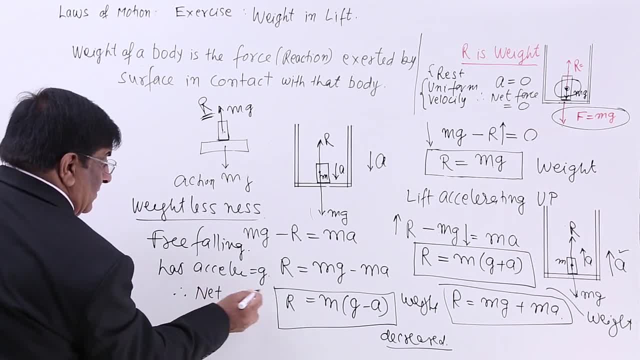 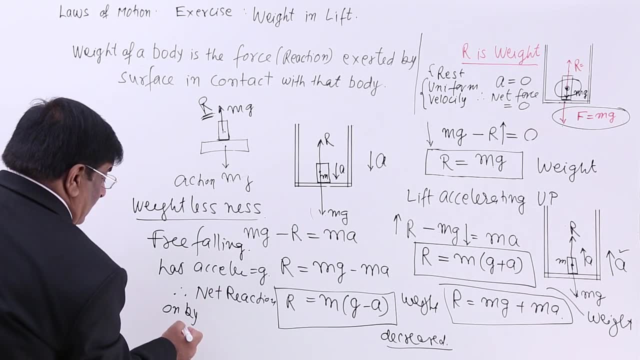 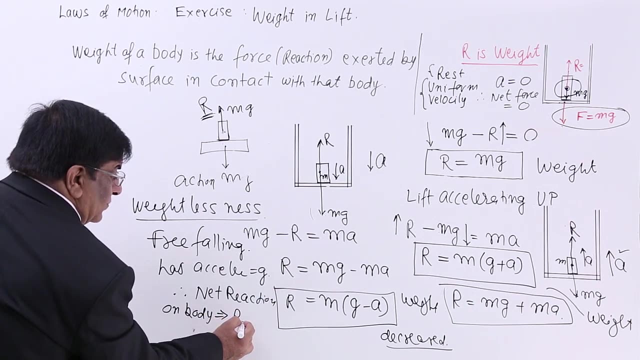 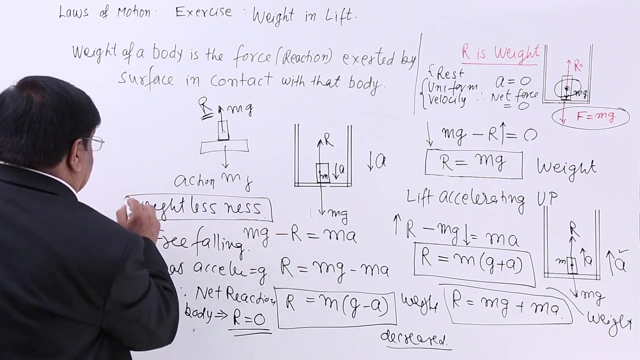 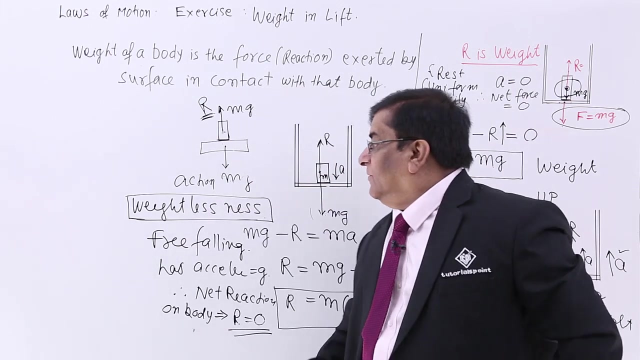 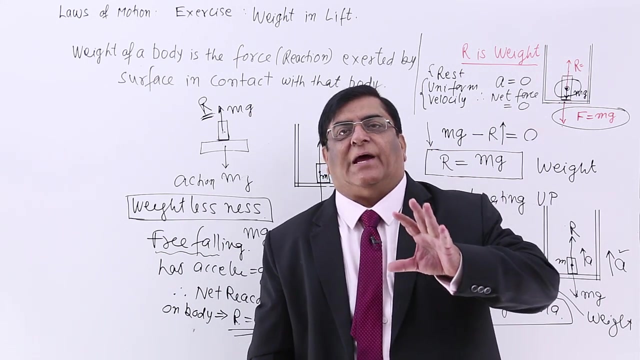 to G. therefore, net reaction on body is R equal to mg minus G 0.. This is weightlessness. and when do we experience it? When we have buggy jumping, when we have free fall- from anything free fall- and that itself is a very strange and out of the world experience, and